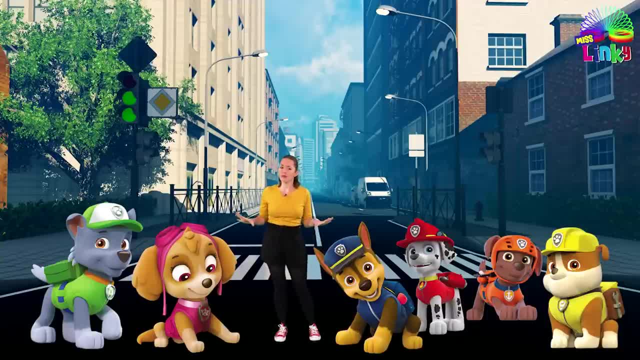 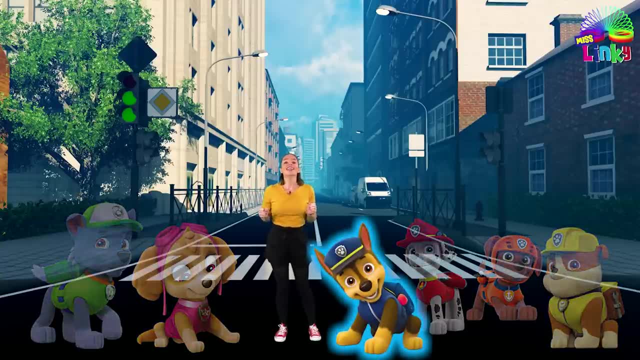 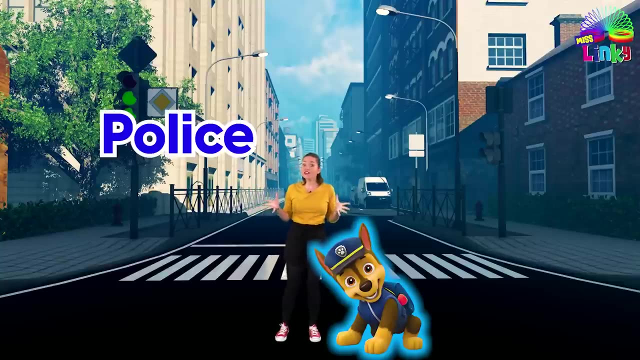 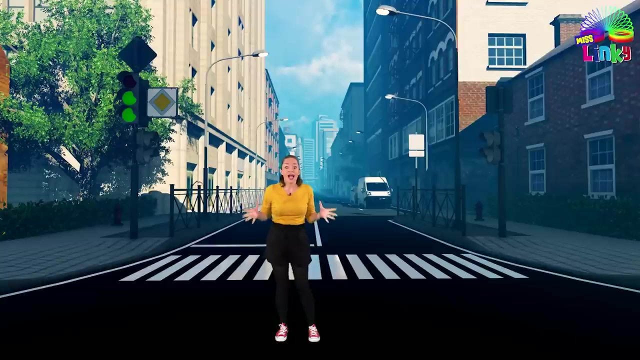 I wonder which Paw Patrol Rescue Pup would usually handle this situation. Do you know? Yes, Yes, That's right, Chase. Chase is a police dog. He's a German Shepherd and his favourite colour is, Yes, Blue. These dogs help us to catch bad guys, and that's what we are going to do. 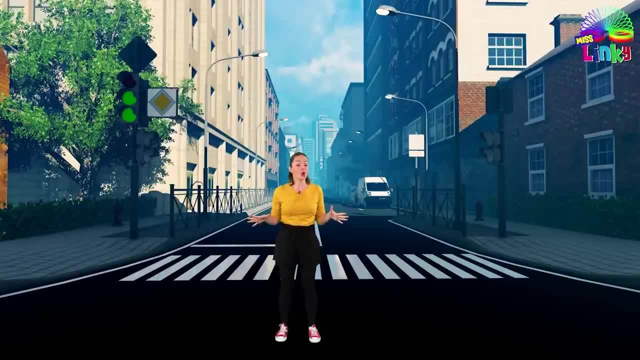 We are going to catch the thief, But first we need to find him. But be very careful because he might throw some things at us. So if you see something coming from the left, we are going to move to the right like this: 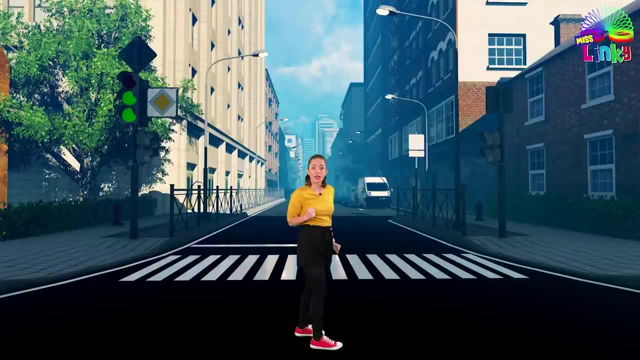 If you see something coming from the right, we are going to move to the left like this. If you see something coming over your head, we are going to duck down like this. And if you see something in the road coming towards your feet, we are going to jump over it like this. 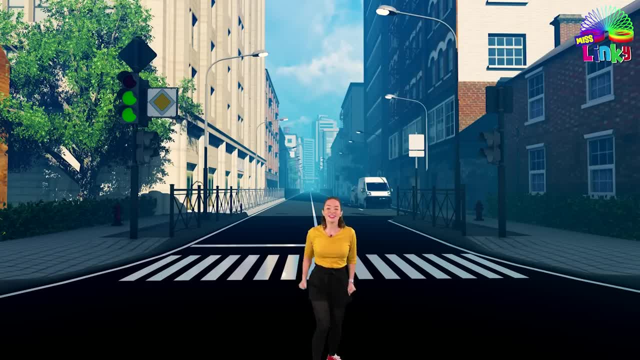 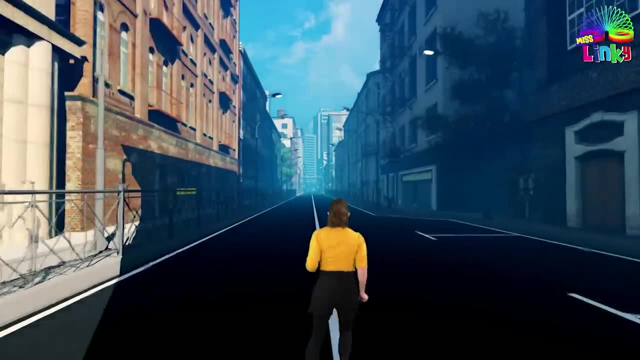 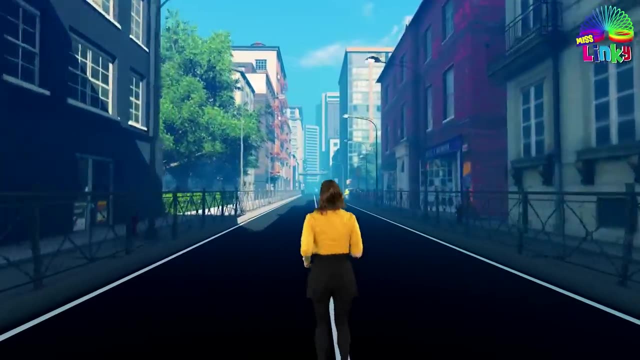 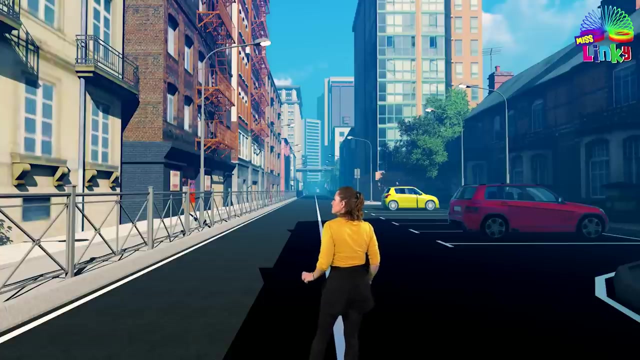 Are you ready to go catch a bad guy? Yes, Great, Follow me, Let's go. I didn't see him anywhere. How about you? No, Maybe he's hiding inside one of these buildings. I wonder which one? What? 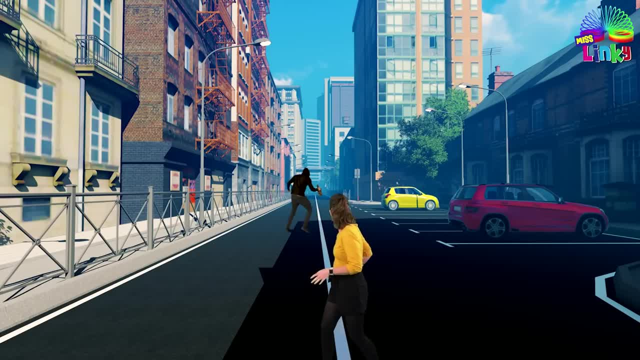 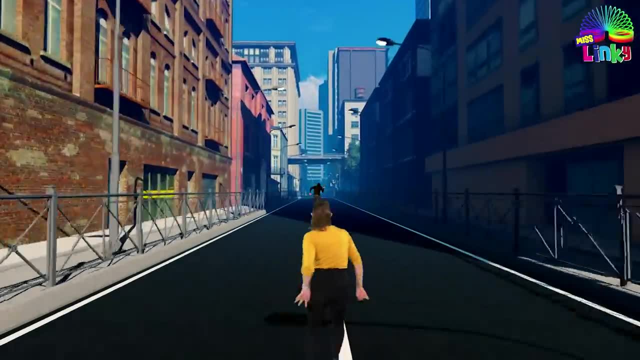 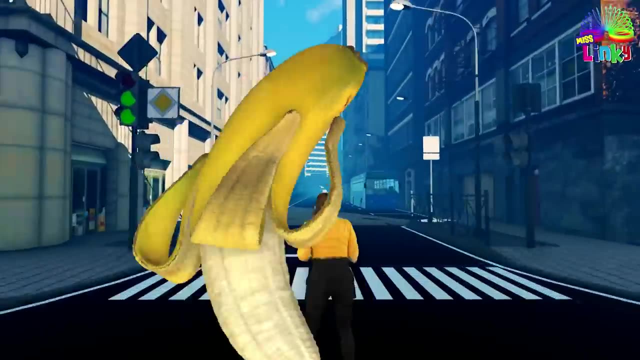 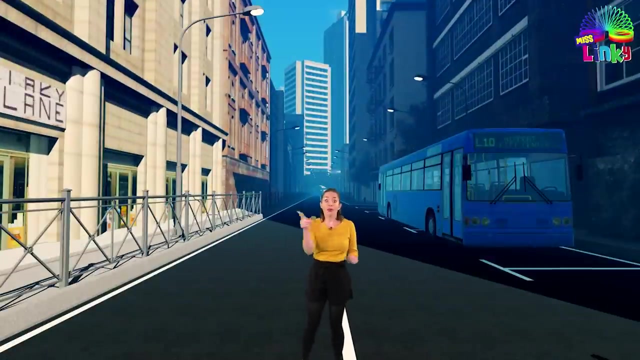 What did you say? He's behind me. Okay, Quick, Let's run Come. I lost him again, But don't worry, He has to be somewhere close. Just keep your eyes open. There he is. Okay. Now we need to run faster. 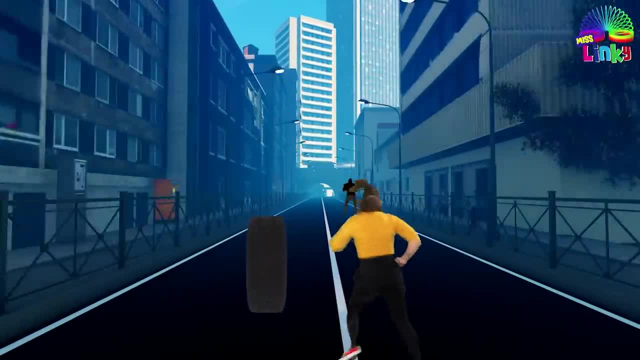 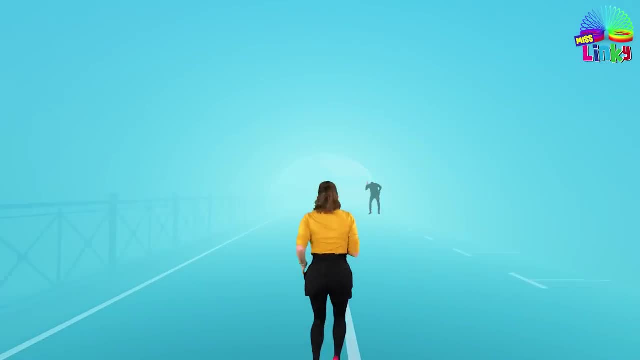 Let's go. Oh, my goodness, It's so misty. I can't see anything, Can you? Oh, no, Okay, We need to be very careful because he has to be somewhere very close. Did you hear that? I heard him. 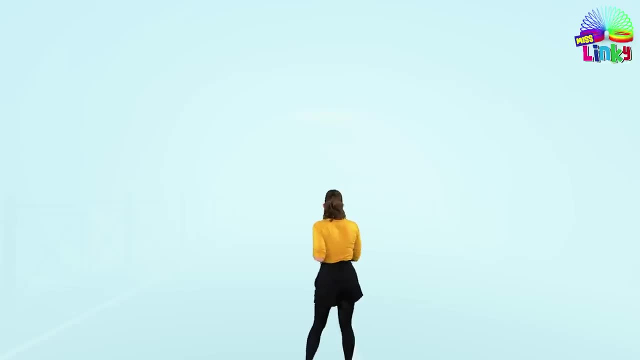 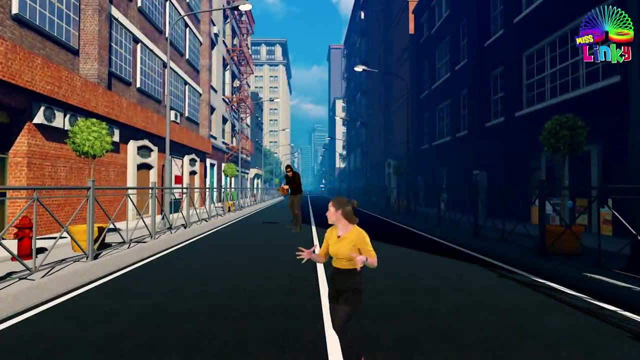 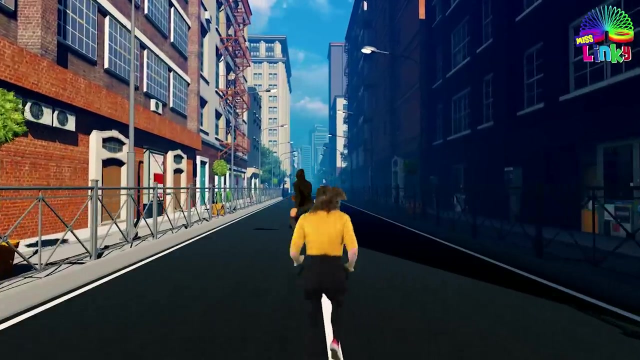 Let's try to get through the mist. That's better. And there he is. Okay, everyone. Now we need to run as fast as we can until we catch the bad guy, But really fast. Until we catch him, Let's go. 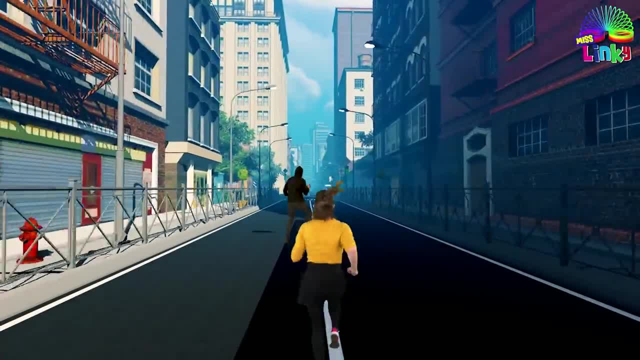 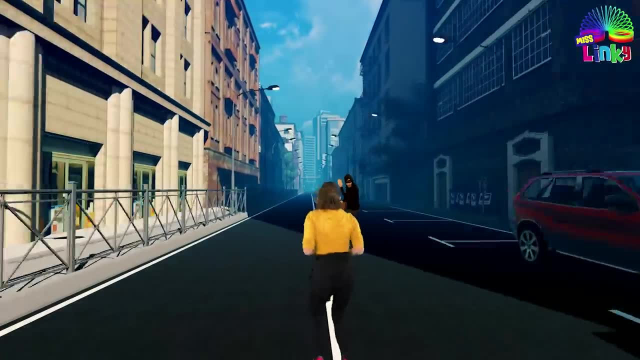 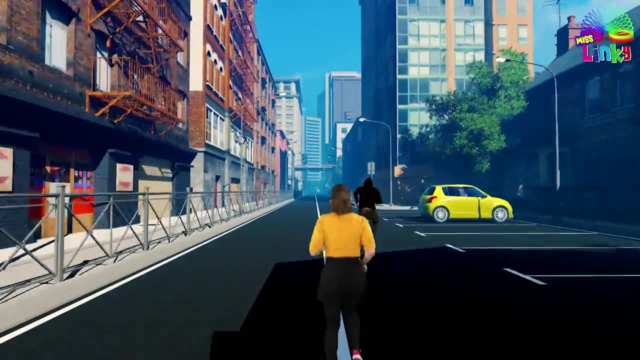 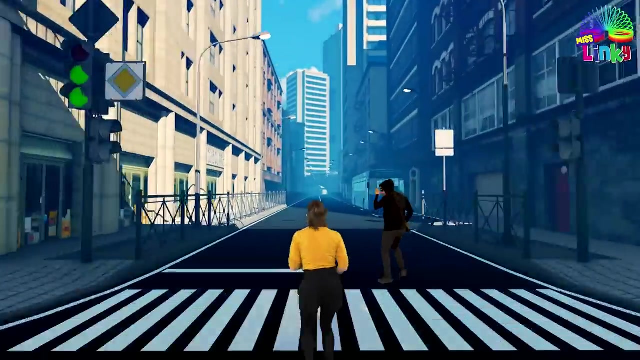 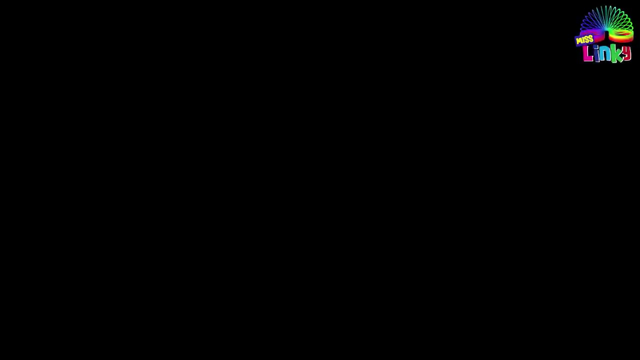 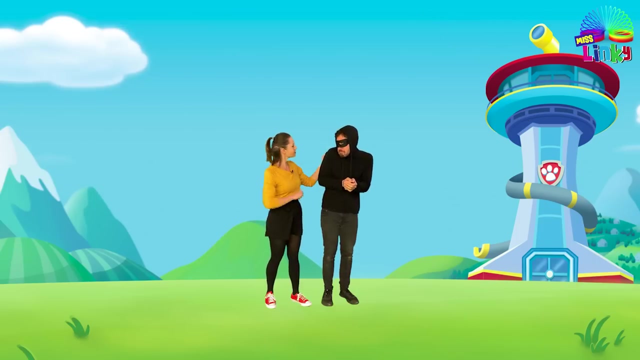 Let's get him. Wait, You did a very bad thing, Mr Thief. It's never a good choice to take things that don't belong to you. I'm sorry, Miss Linky. I hope you learned your lesson. Now go think about what you did. 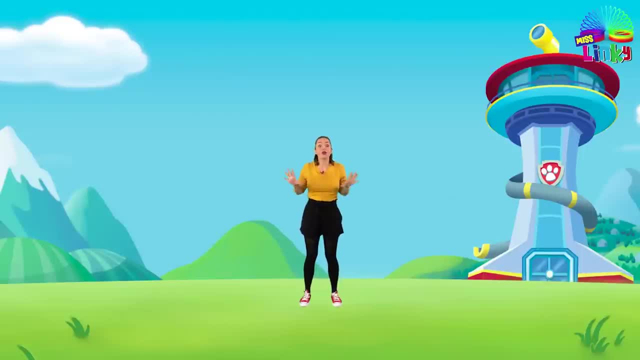 Okay, everyone, Now we are going to practice our air rescue pup skills just like Skye. Skye is a cockapoo kind of dog and her favorite color is pink. Skye is a pilot. Pilots fly things like airplanes. 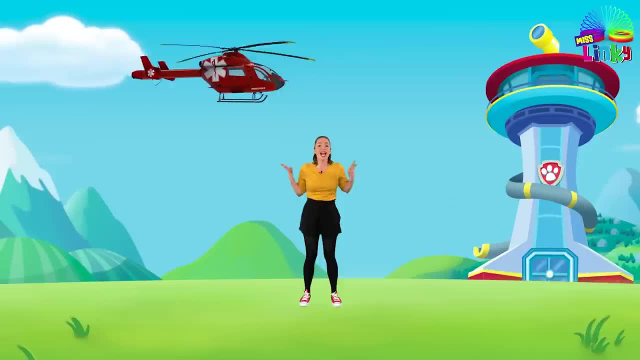 And helicopters, So we are going to practice our helicopter skills. Helicopters have big blades that spin around really fast, So we are going to use our arms as blades. So put out your helicopter blades. That's it. Keep your arms up. 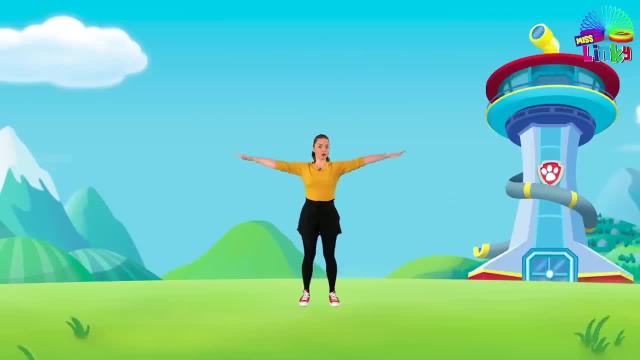 And now we are going to spin our blades in small circles. Do it with me. Good job, Keep going. Now let's make it A little bit bigger. Good, Even bigger, Even bigger, Yes, And now as big as you can. 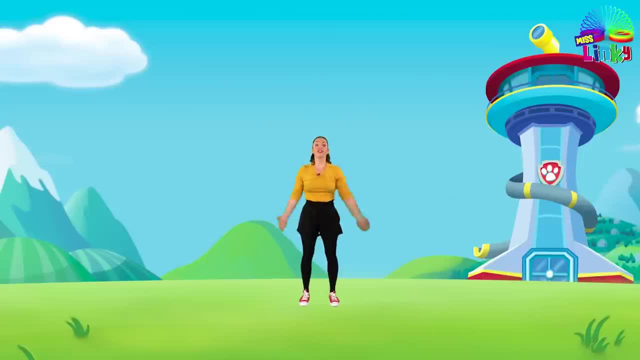 Good, Keep going. Now let's do it for ten counts. Count with me One, Two, Three, Four, Five, Six, Seven, Eight, Nine, Ten. Good job, Keep your arms up. Now we are going to spin it backwards. 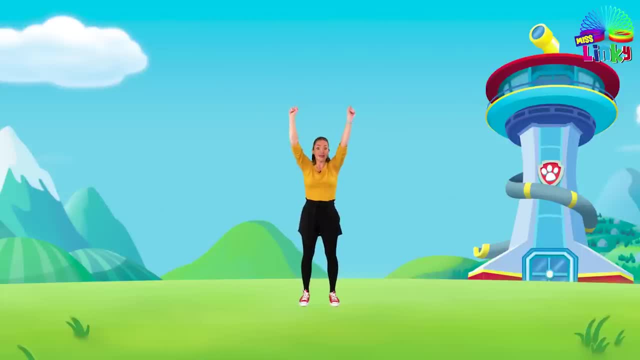 And we are going to count backwards too. From ten Ready, Let's go Ten, Nine, Eight, Seven, Six, Five, Four, Three, Two And one Whoo. my arms are tired now. Good job, pilot. 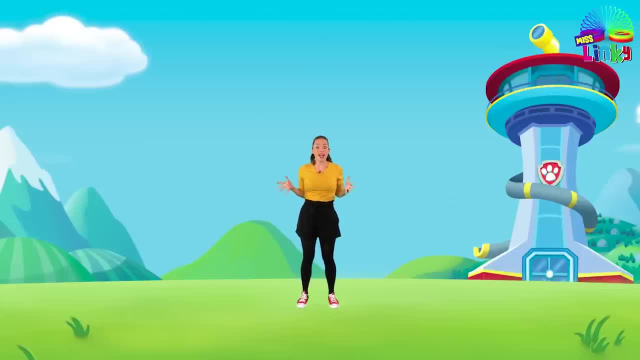 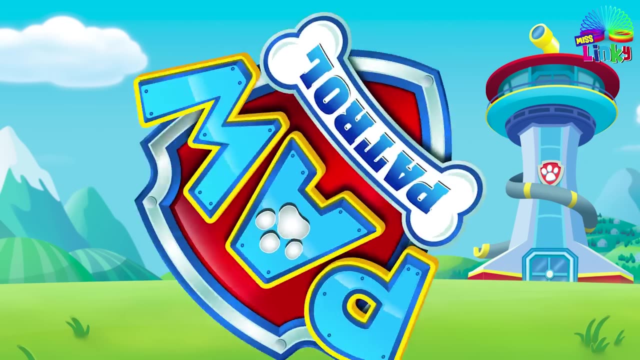 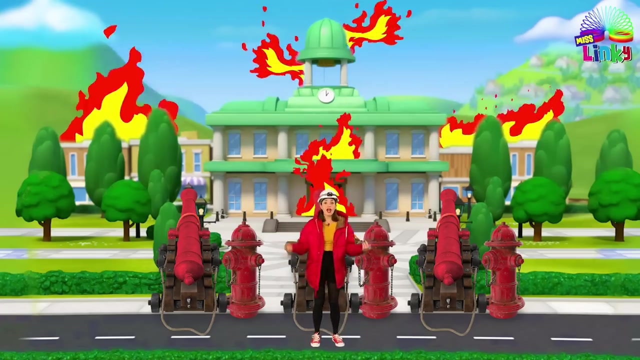 Don't go anywhere, because next we are going to play a fun game where we will practice our fire fighting skills, just like Marshall. Watch this game. Oh no, The down hall is on fire and we need to help to put out the fire, just like Marshall. 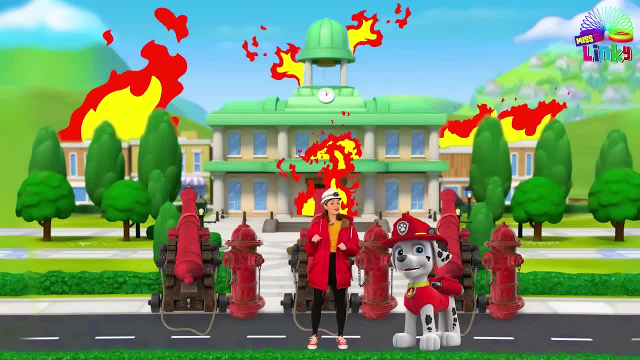 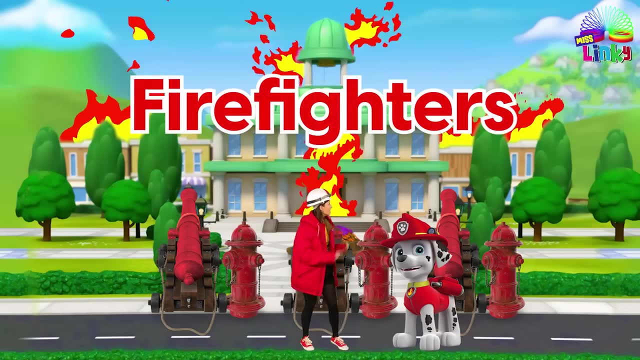 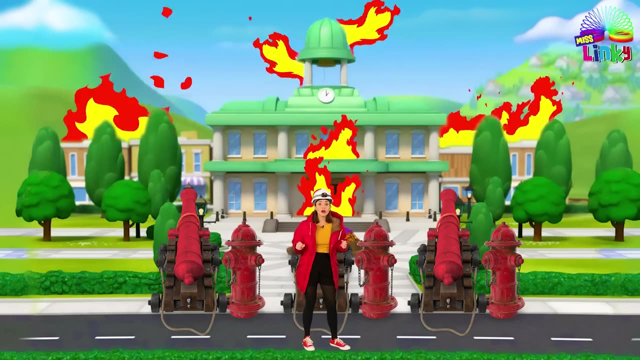 Marshall is a Dalmatian kind of dog and his favorite color is red. Firefighters put out fires and we need to put out these fires. So when you see fire coming out of the building on the right-hand side, we are going to shuffle to the right. 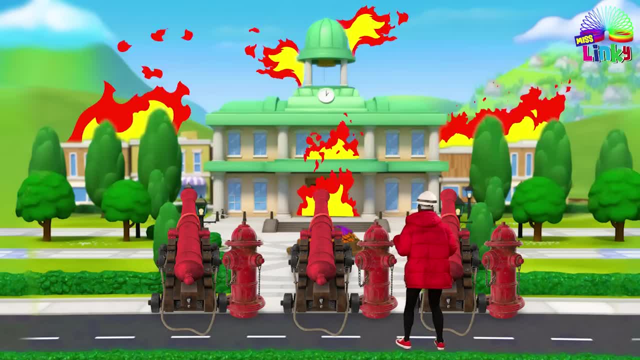 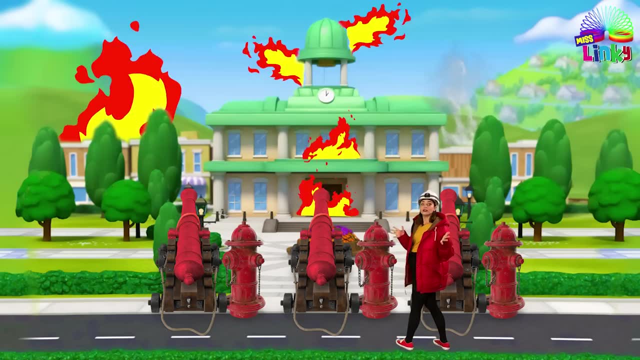 Shuffle with me, Shuffle, shuffle, shuffle, shuffle. And then we're going to squat down like this: Squat down and activate the water cannon When you see fire coming from the left-hand side of the building. we're going to shuffle to the left. 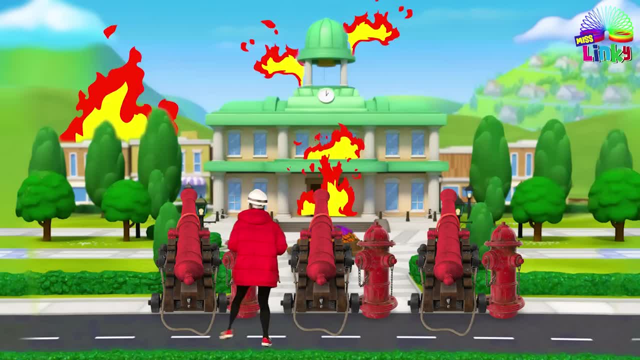 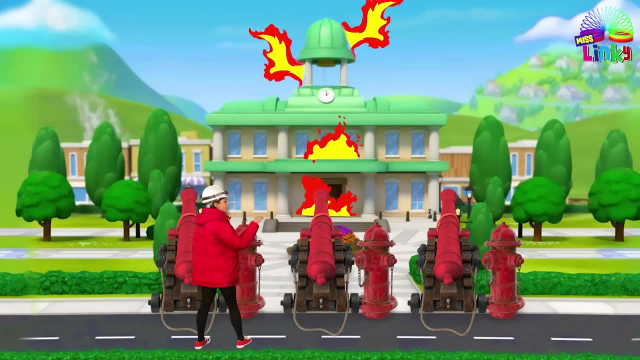 Do it with me: Shuffle, shuffle, shuffle, shuffle, shuffle, shuffle, Squat down and activate the water cannon When you see fire coming out of the middle part of the building. we're going to shuffle to the middle, Let's go. 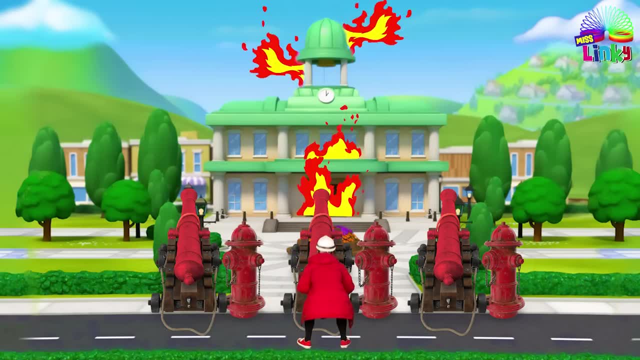 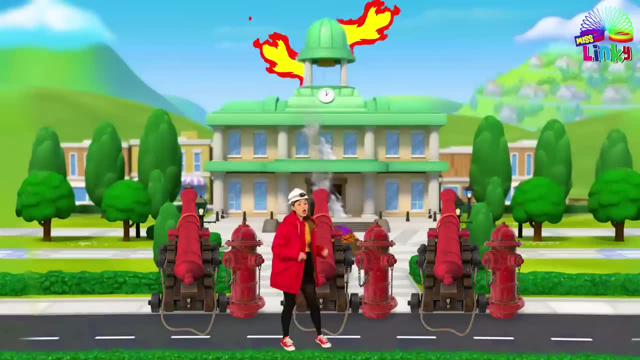 Shuffle, shuffle, shuffle, shuffle And squat down To activate the water cannon. When you see fire coming out of the top part of the building, we need to call Skye and Zuma to bring water with a helicopter. So we are going to do five firefighter star jumps. 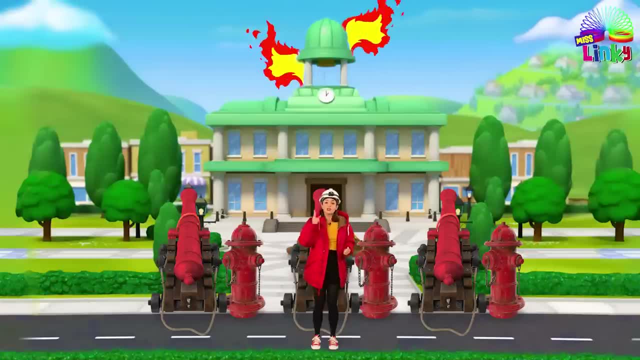 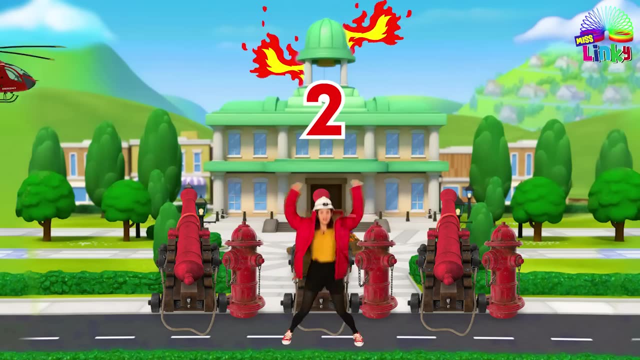 to signal to them that we need air support. So let's do five firefighter star jumps together. Let's go One, two, three, four, five, Perfect, And that is how we are going to put out all the fires. 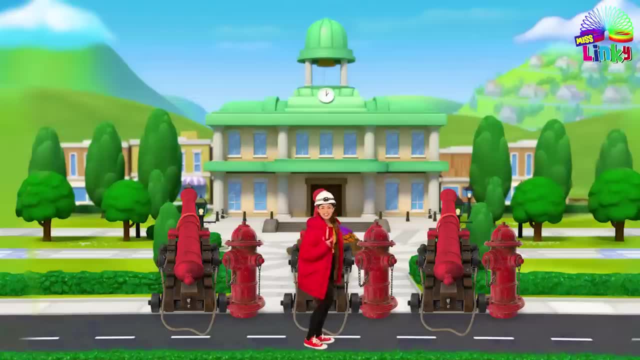 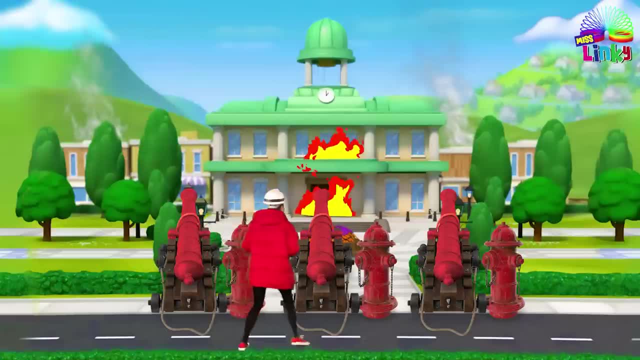 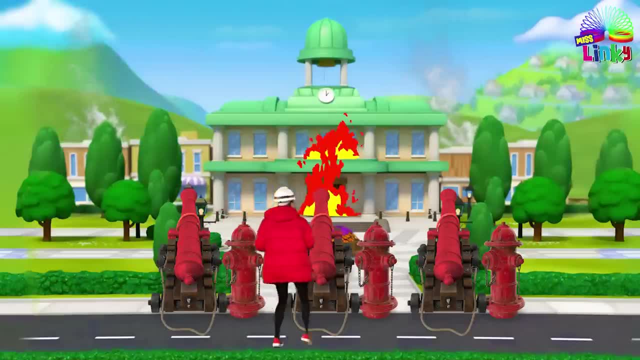 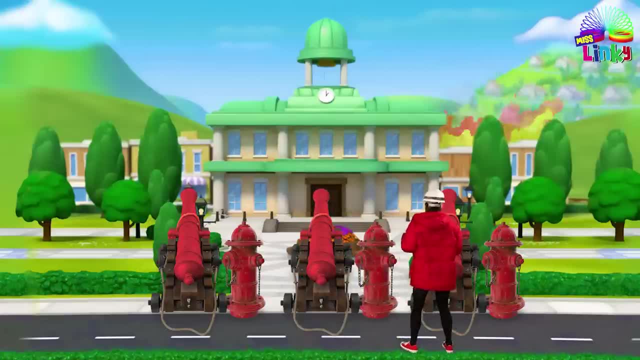 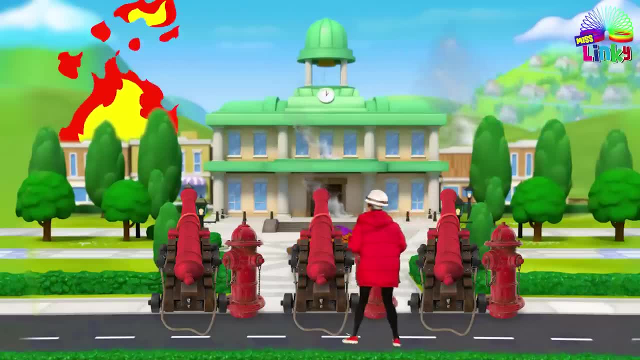 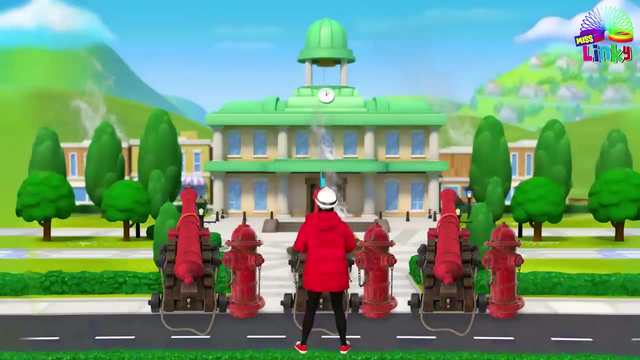 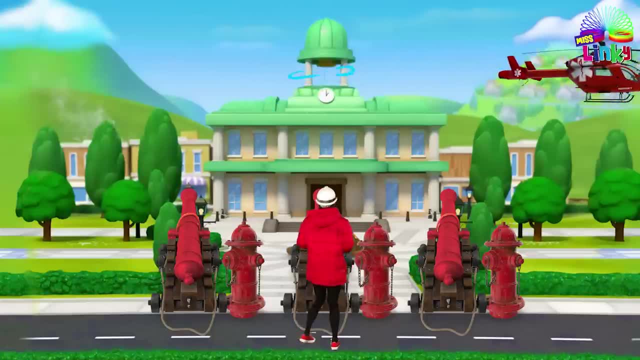 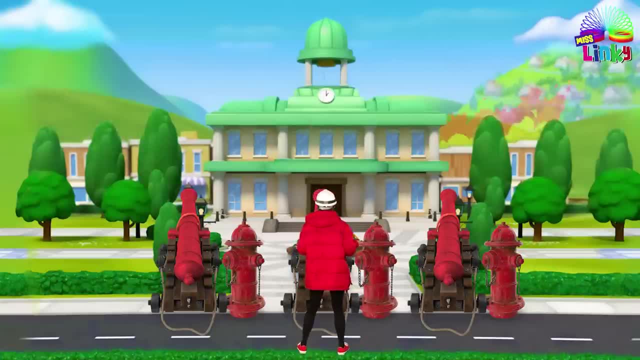 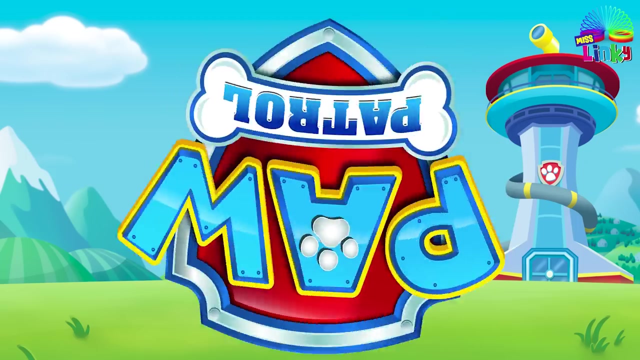 We're almost there. One, two, three, four, five. Yay, One, two, three, four, five, Yay, We did it. We put out all the fires. Well done, Shoo-wee. That was a lot of fun. 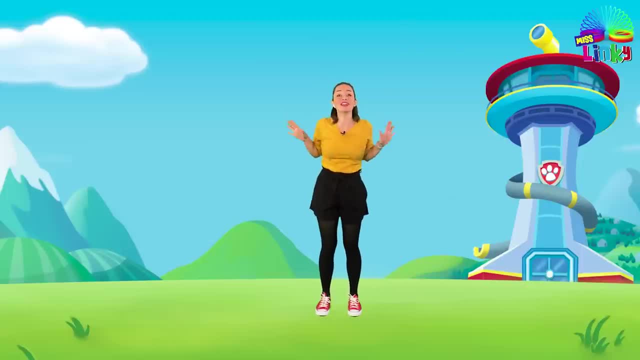 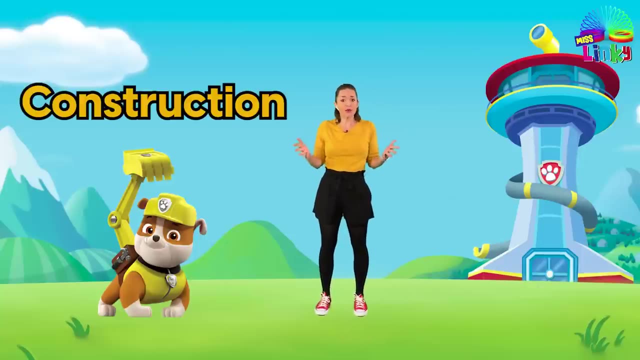 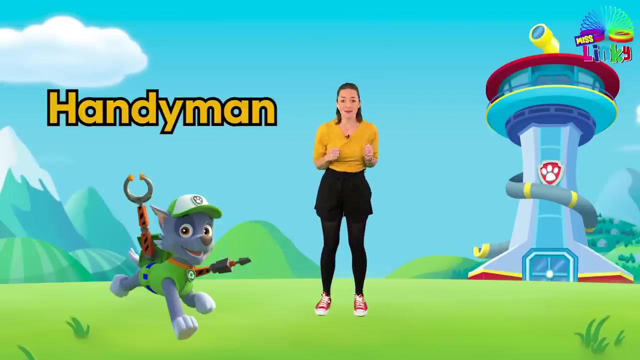 But stay right where you are because this is going to be even more fun. Rubble is a construction pup and he is a bulldog. Construction pups like to build things. And Rocky is a mixed breed dog and he is a handyman, Which means he likes to fix things. 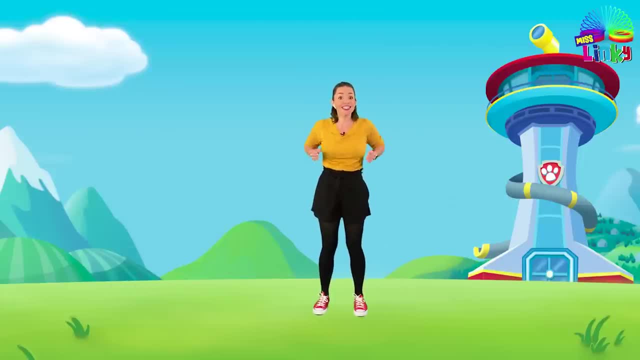 So we are going to practice our building and fixing skills with the Rocky and Rubble dance. So let me teach you the dance moves When you see a picture of bricks. we are going to do these two moves. First, we're going to smear the concrete. 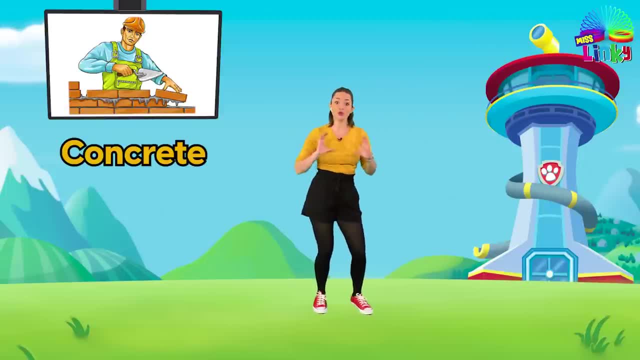 Smear the concrete, And then we're going to lay the bricks, Lay The bricks. Do it with me: Smear The concrete, Smear The concrete And lay The bricks. Lay The bricks, Lay The bricks. 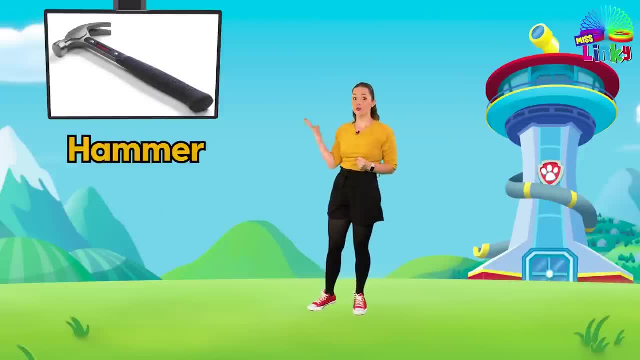 Perfect, Okay, the next move is the hammer. So when you see a picture of a hammer, we're going to go: hammer, hammer, Hammer, Hammer, Do it with me. That's it Perfect, Perfect. a picture of the screwdriver: we're going to do the screwdriver move. So we put our 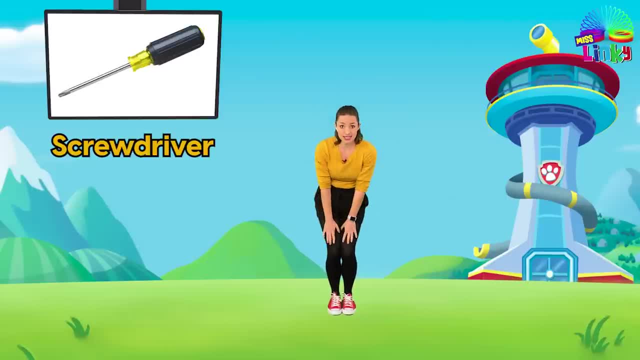 knees together, we put our hands on our knees and then we make a circle with our knees. That's it. So make a circle with your knees, just like a screwdriver- Awesome. The next picture is a wrench. When you see the picture of the wrench, we're going to do this move. 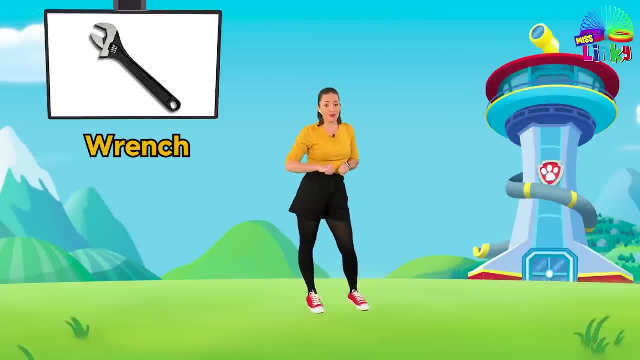 So pretend like you're holding a wrench with both your hands and we go this way, that way, this way, that way. Try it with me. This way, that way, Good, That way, Perfect. And the final move is the paintbrush. So when you see the picture of the paintbrush, we're going. 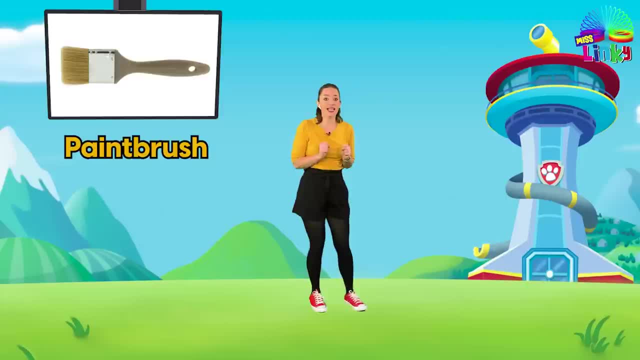 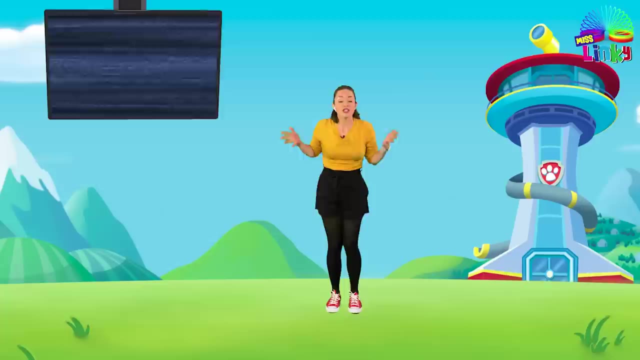 to use our hands as paintbrushes and we're going to paint like this: Paint And paint, Paint And paint. One more time, Paint And paint. Amazing, I think you've got it. So are you ready to do the Rocky and Rubble dance? Yes, Perfect, Let's get started. Okay, now. 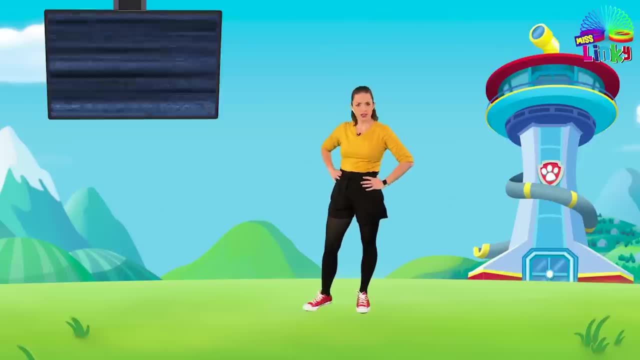 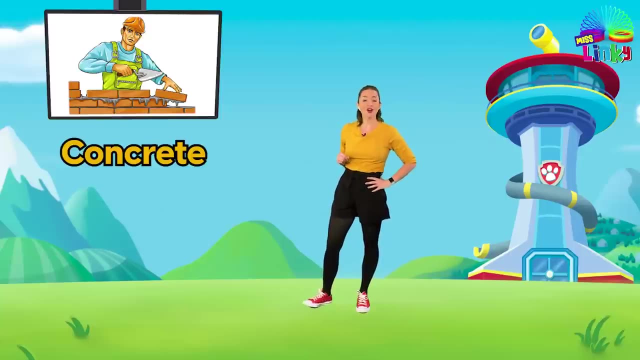 listen for the beat. Let me see you tap. Okay, Elbow, left foot, right foot, your foot, Yes, Okay. First move is the concrete. Let's go And concrete And bricks And bricks, Concrete, Concrete, Bricks, Bricks, Smear, the. 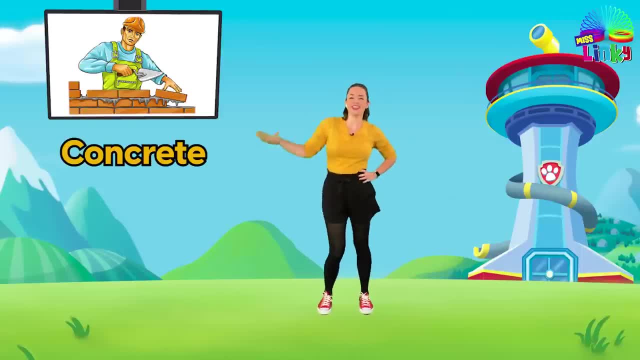 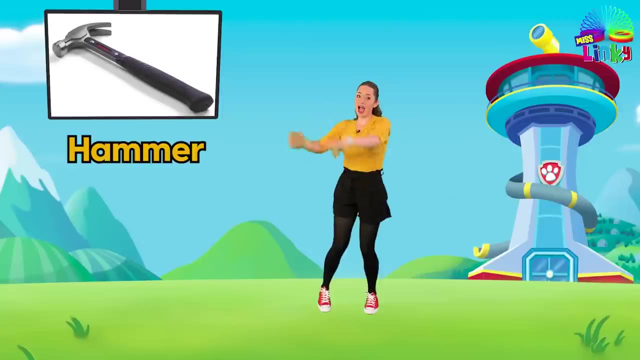 concrete, Yes, Bricks, bricks Out of the box, bricks Out of the box. I do need more work and light on the floor, guys. Yeah, Bricks, one more time. Concrete, Concrete, Bricks, Bricks, Hammer, Hammer, Hammer, Hammer, Hammer. 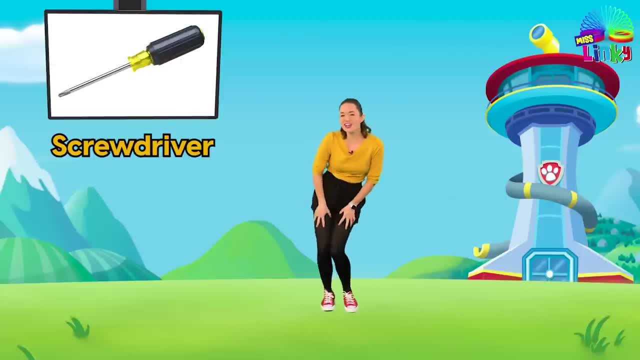 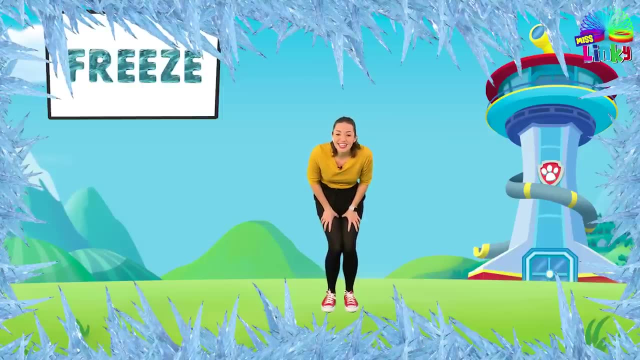 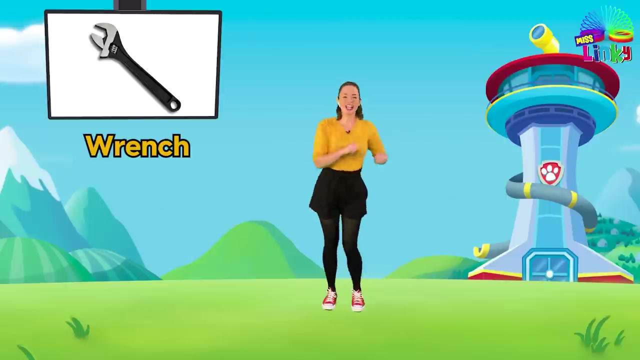 And screwdriver Freeze. Stay where you are, Here we go. Time for the wrench. Yay, The wrench, Keep going. You're doing great. And now paintbrush, Paintbrush, Paintbrush, Paintbrush. Keep painting, Painting, Painting. 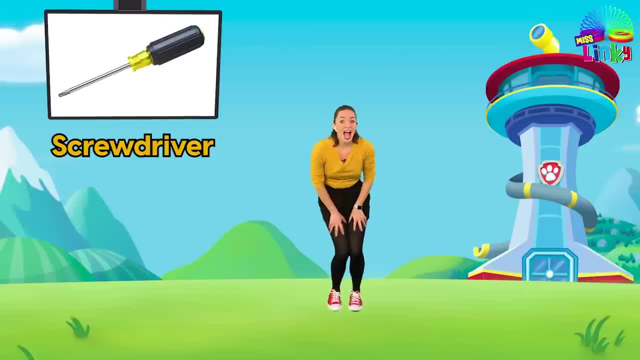 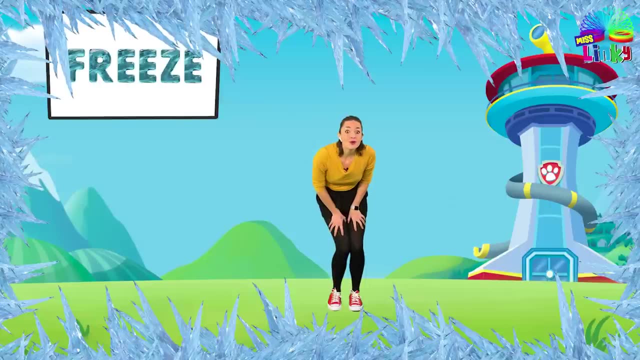 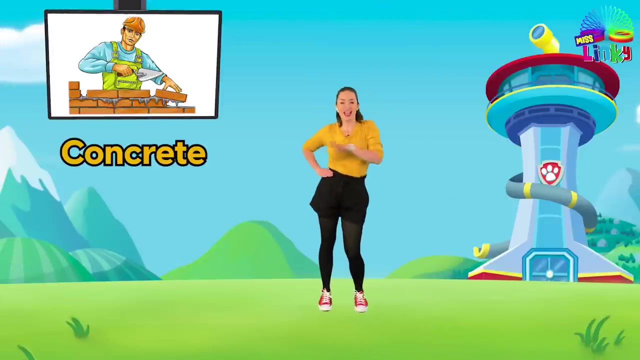 And screwdriver And freeze, Don't move. You were amazing. Stay frozen. And when the music plays again, we are going to do the moves even faster. Are you ready? Yes, Let's go. Alright, And concrete, Concrete Bricks, Bricks. 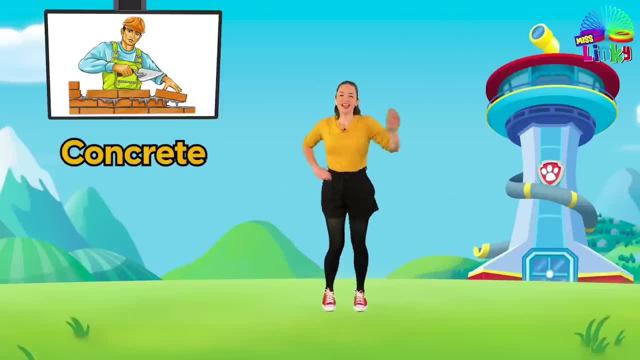 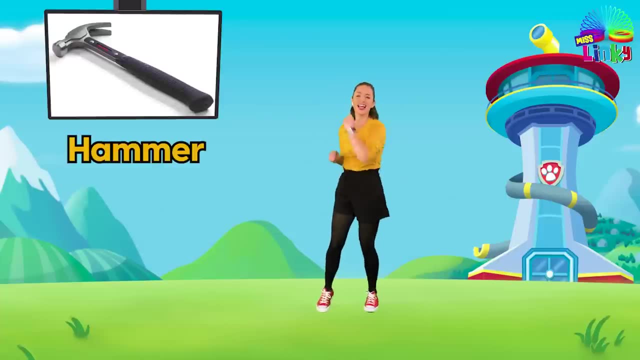 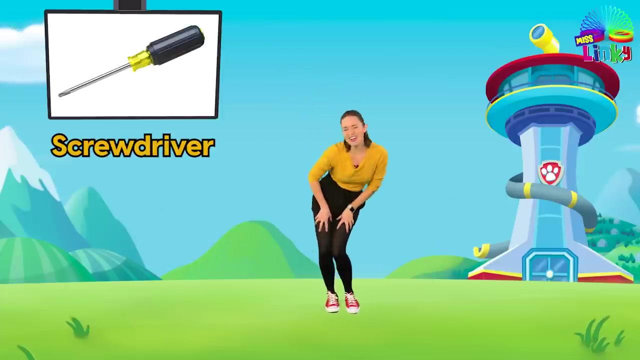 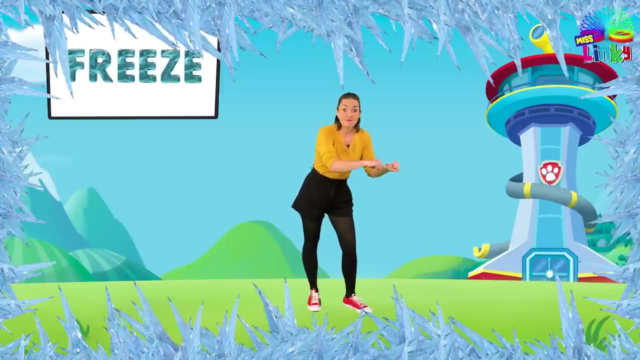 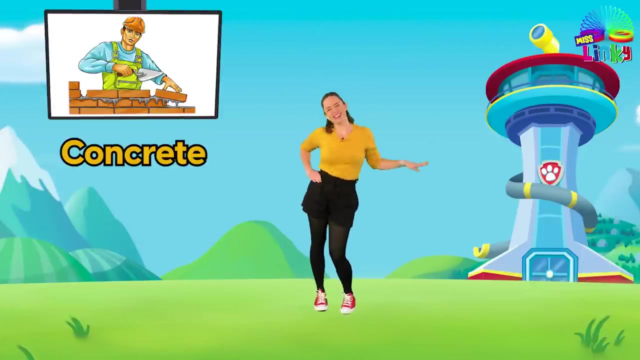 And concrete, Concrete, Bricks, Bricks, Hammer, Hammer, Paint, Paint Screwdriver. Good job And rich, Rich, Well done. Good job And freeze, Stay frozen And ready For the concrete, Concrete Bricks, Bricks. 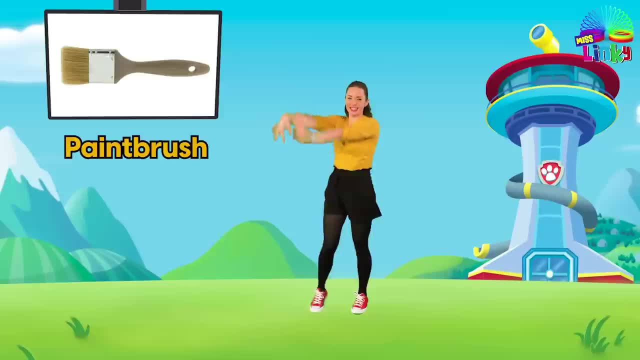 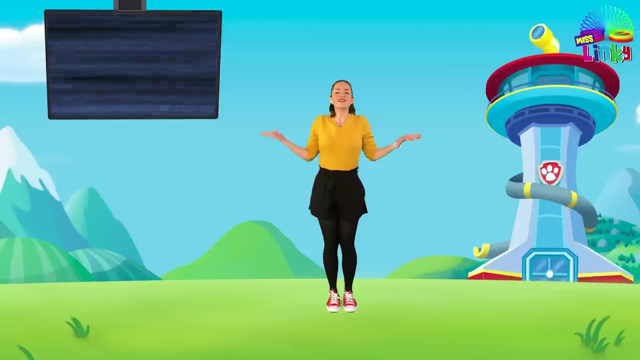 Frame Frame Screwdriver- Frame Frame Screwdriver- Range Hammer Hammer Frame noses Hammer Hammer czasu Fade away near the finish. Top nicht And finish. Wow, That was amazing. I love the Rocky and Rubble dance. 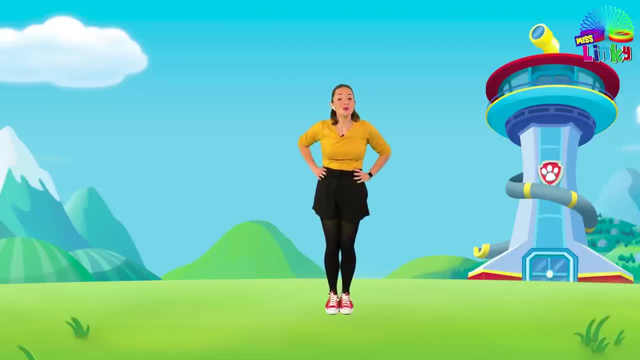 How about you? Yes, Well, you were incredible. I loved your dance moves And we have completed all three dances. Fifty year old And you, You, Hey And I- I'm so excited- completed our Paw Patrol Rescue Pup training. You were amazing. 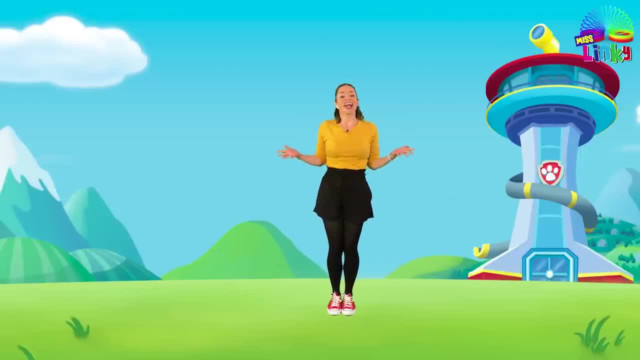 Congratulations. Thank you so much for training with me today and I'll see you again next time. Bye.